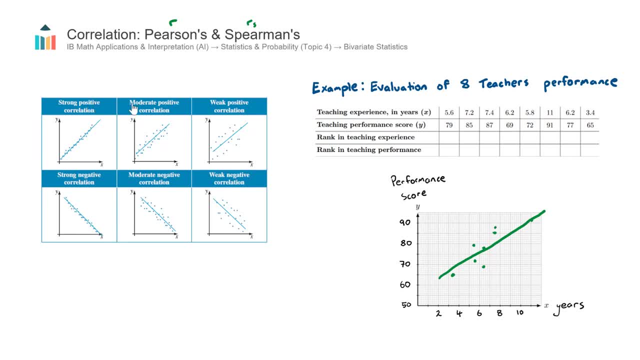 direction. so you can see here, the top row here are all positive. so the line is sloping upwards. and then the proper way to think about that is: as the independent variable increases, so does the dependent variable. so an example of that is, let's say, the growing, the height of a growing child. as the child increases in age, their height. 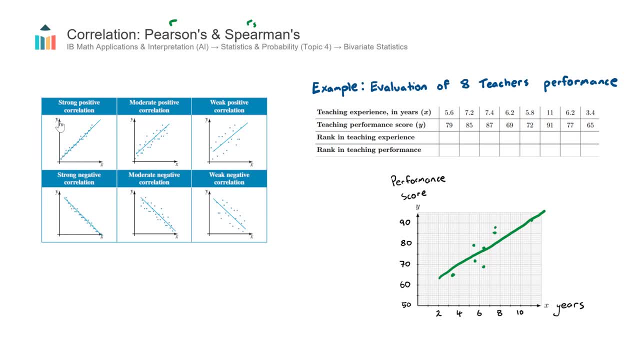 also increases, so both variables increase. conversely, these three bottom negative correlations. so the line of best fit or the trend line is going downwards. an example of that would be, say, the temperature of the day. so as the temperature increases, and maybe the number of coffee sold was usually on hot days, coffee isn't sold as well, so the number of coffees would. 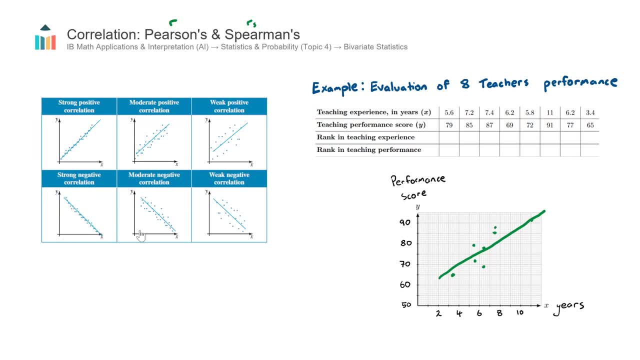 actually decrease as the temperature increases. so these three bottom ones here examples of negative correlation. so we have talked about there the direction, either positive or negative. the second description is the strength, and the way to think about that is how close are the data points to the line of best fit. so these two left hand ones here, both strong, positive and strong. 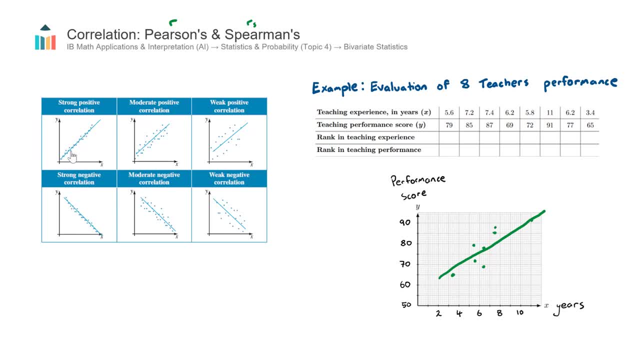 negative, the. the data points are very, very close to each other. so the line of best fit is going close to the line. so in other words, the line of best fit really follows the trend very closely. the middle two here we call moderate, so the data points are kind of close to the line, the trend. 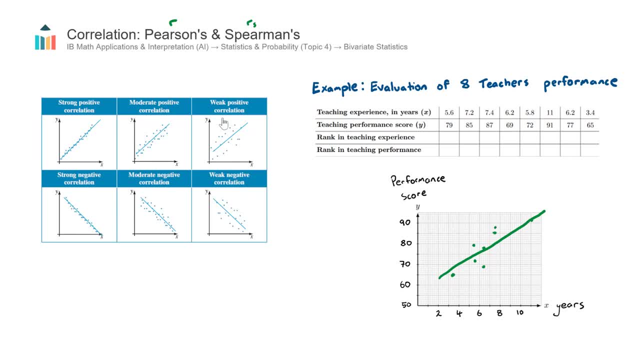 line kind of summarizes it nicely and the two right ones here, both weak positive and weak negative. the data points are quite a long way away from the trend line and and the the, the line of best view, doesn't actually sort of summarize the trend very well. now, the value that we use. 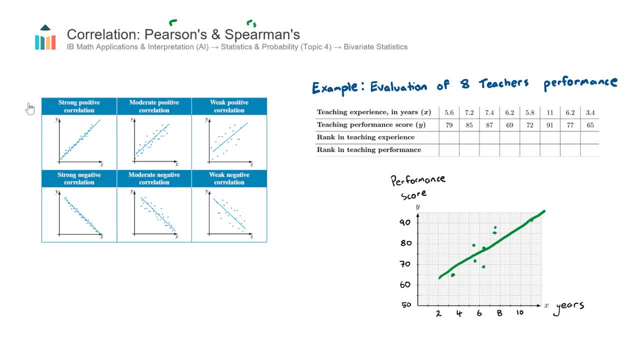 to actually determine that that trend is actually sort of similar, the kind of voir on hi every step and the strength is an R value called the Pearson's product moment correlation coefficient. So this R value here Now strong correlations are anywhere. there's sort of different schools of thoughts here. 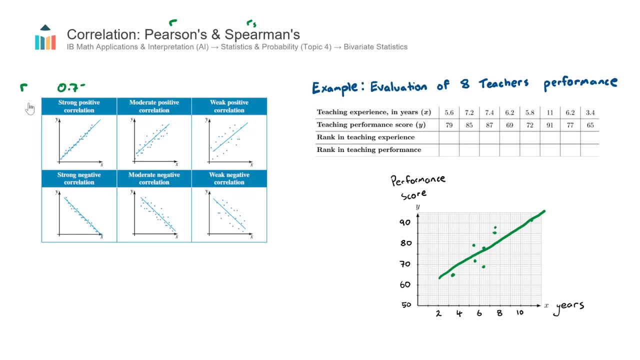 but basically anywhere between about 0.75 and one where one is the strongest perfect correlation that would be considered strong, Moderate would be between about 0.5 and 0.75 and weak would be about 0.1 to about 0.5.. 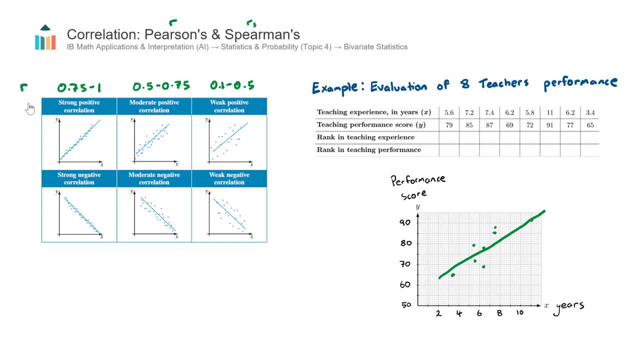 And if you had a correlation of zero, there would actually be no correlation between the variables. On the negative side, exactly the same, but just reverse the sign, So between negative 0.75 and through to negative one, that would be strong negative. 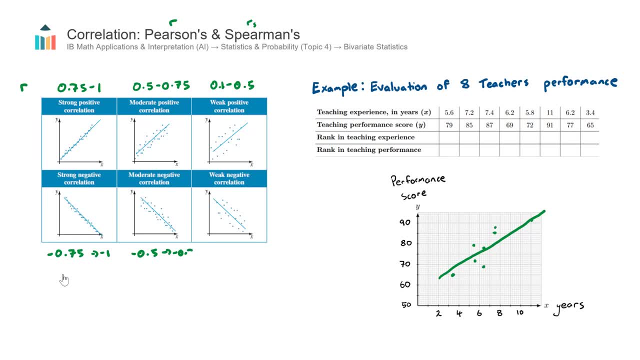 Negative 0.5 all the way to negative 0.75 would be moderate negative, And then negative 0.1 all the way through to negative 0.5 would be weak negative. Okay, so let's go ahead and actually find the R value. 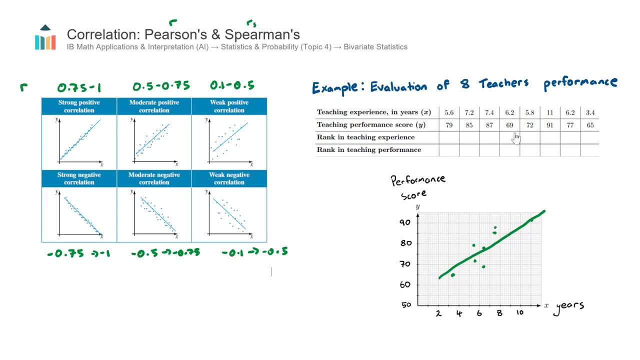 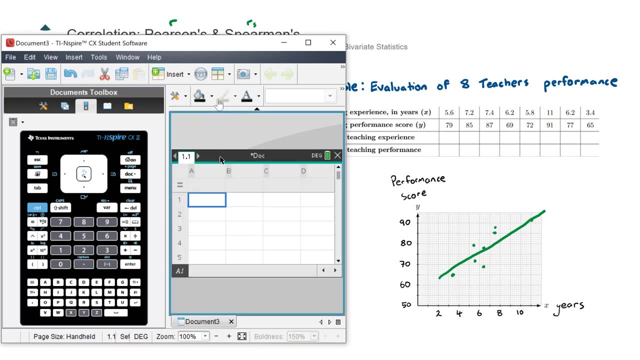 for our example here We have eight data points and we're going to use our calculator to actually find the R value. Okay, we bring the calculator up, we go to this green statistics icon here and we enter in this data, And I'll do this fairly quickly. 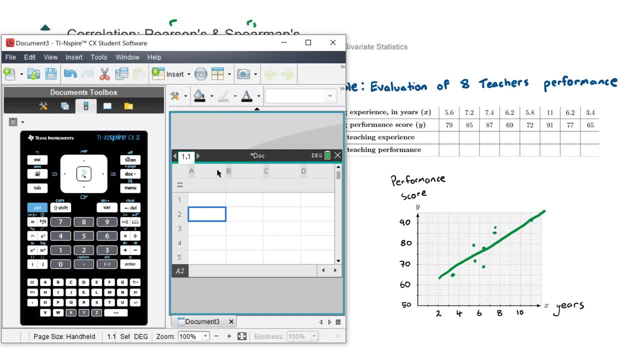 because there's plenty of questions to practice on in the question bank. but we label the first column, our independent variable, we label our second column, our dependent variable, and then we go ahead and enter the data points. So the first one is 5.6 years taught. 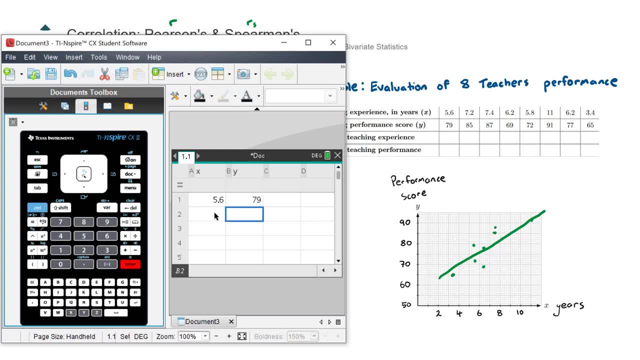 and with a performance score of 79.. Now we'll go ahead and enter the next seven. Okay, there are the eight data points entered. Let's go to the top of the next column and perform a two variable statistic calculation. So we go. menu number four statistics. 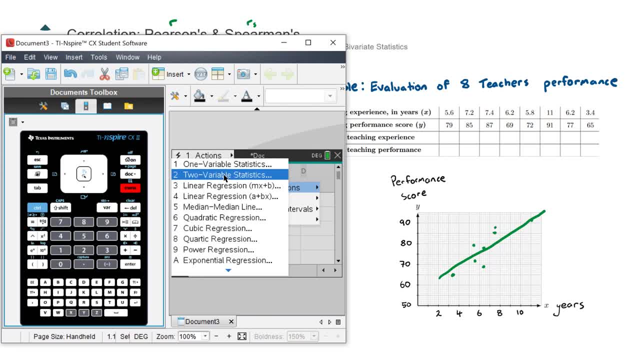 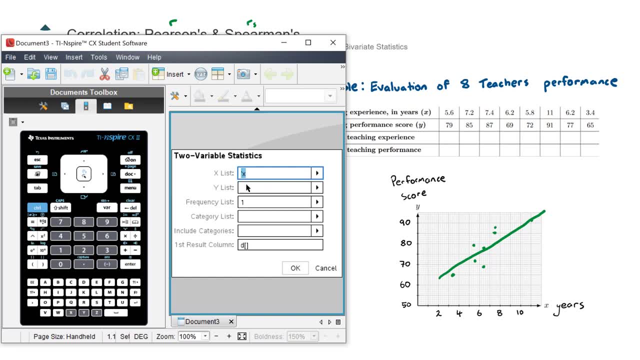 number one stat calculations and this number two here, because we do have two variables here: number of years teaching and teacher performance score. The X list: we select X for the first column. The Y list: we select Y hit okay. 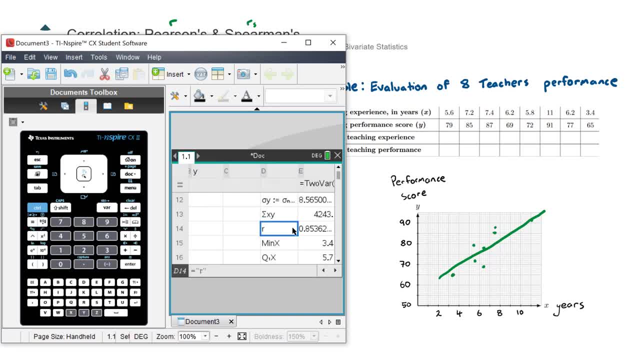 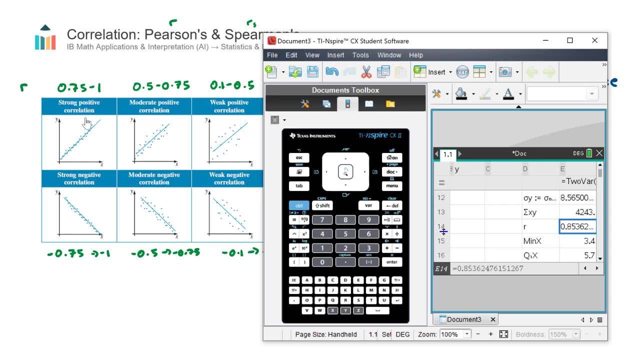 And if we scroll down we get our R value down. So our R value is 0.854, rounded to three sig. fig, And you can see here that that would be described as strong positive correlation. So in other words, there is a strong positive relationship. 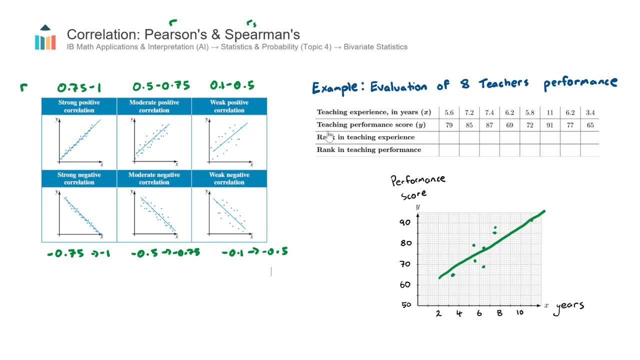 between the number of years a teacher has taught and their associated teacher performance score. Okay, so that's the Pearson's product moment correlation coefficient R. Let's now talk about the Spearman's RS. It's essentially the same, but instead of 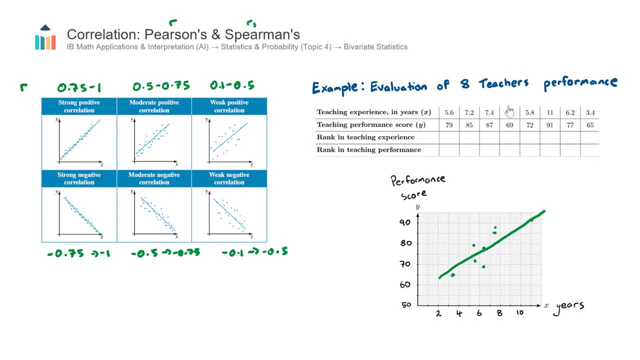 it measuring against the raw data here. instead, it actually measures the same correlation, this value here, that we found in our calculator, the R value, but instead of it being on the raw data, it's actually on the ranks instead. Now, what do I mean by ranks? 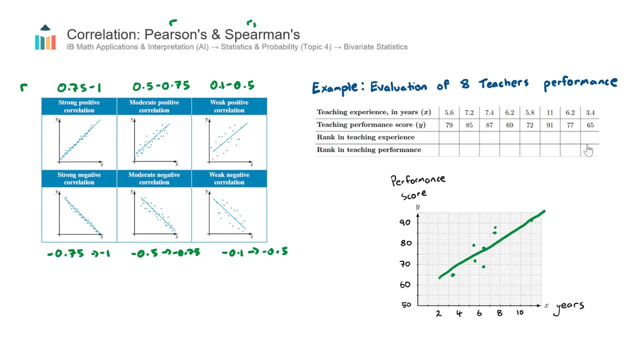 It means that- and this is what I have these two empty rows here for- I'm actually going to rank my teachers in this case in order from one to eight, where you can actually choose whether it's ascending or descending. I'm gonna go with descending. 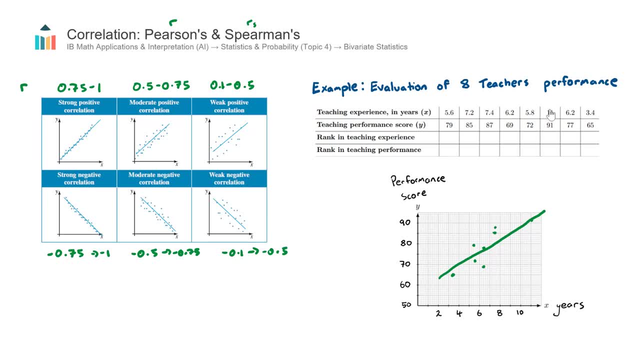 which means the highest number of teaching years will receive a rank of one. So that's this one here, All the way down to the lowest, which is this last teacher here. this last teacher will have an eight, And likewise for the teacher performance score. 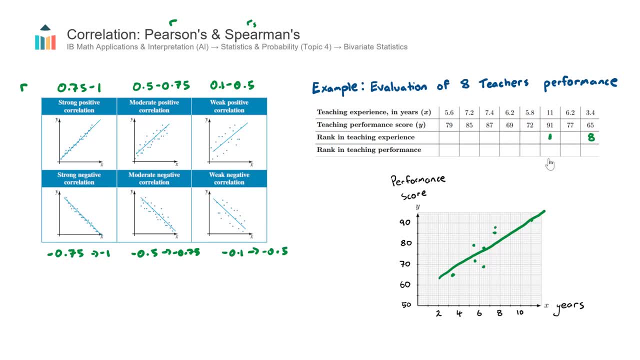 the highest performance score will get a one- this one here, all the way down to the lowest teacher performance score, which in this case here is also this eighth teacher. So I'm just gonna pause the video now and enter the remaining values. Okay, so there are the ranks there. 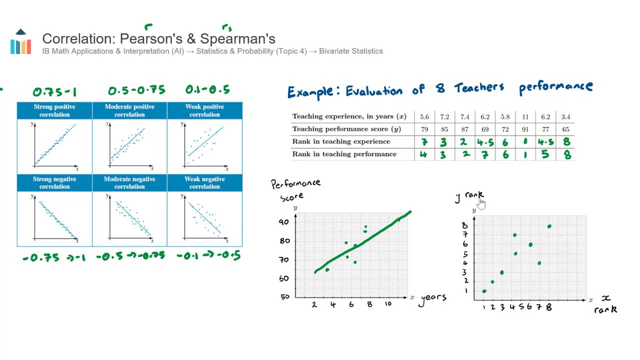 And then I have plotted the actual ranks, So not the actual raw data itself: the ranks of the teacher years and the teacher performance score. So, for example, this one one here represents this teacher here who has been teaching for 11 years and had the highest performance score. 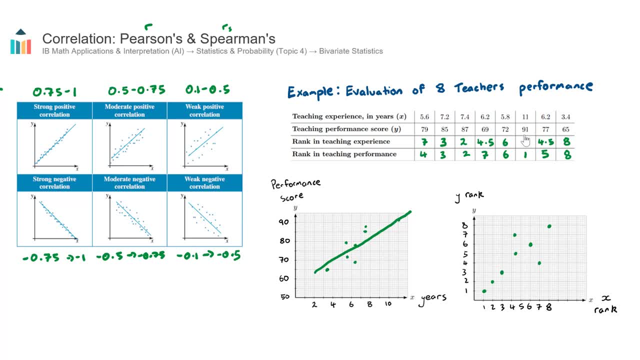 So this teacher had both the most number of years taught and the highest performance score, So that the teacher here is this one one, And likewise this right-hand teacher had the least number of years taught. So they had a ranking of eight out of the eight teachers. 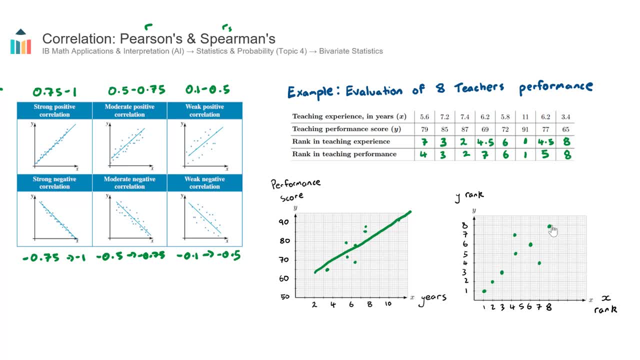 and also the lowest performance score, which is also an eight, and that's this eight eight here. Now, it wasn't a perfect correlation. It didn't go one, one, two, two, three, three. There was a bit of a jumble here in the middle. 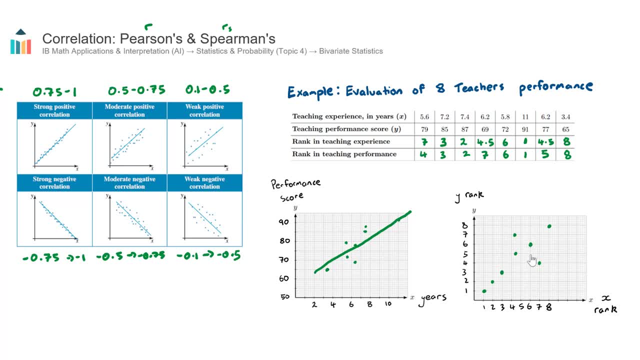 So the Spearman's rank correlation coefficient is actually a measure of the correlation of the ranks themselves. So if I was to overlay a line of best fit here, something like that, again it's asking you a question: well, how close are the data values to this line? 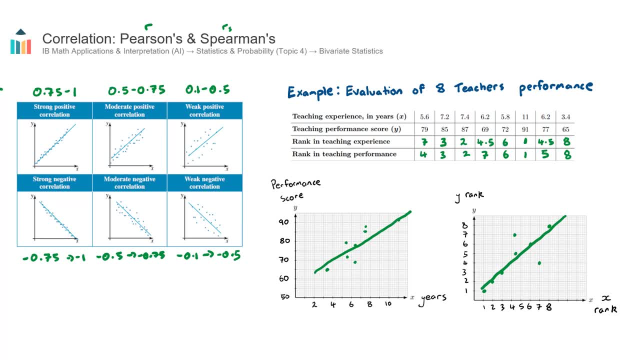 How strong is the correlation? Now to find RS, it's actually the same process as the process we did to find the Pearson's product correlation coefficient, but instead on the calculator we actually enter the ranks instead, And that's what I have done there. 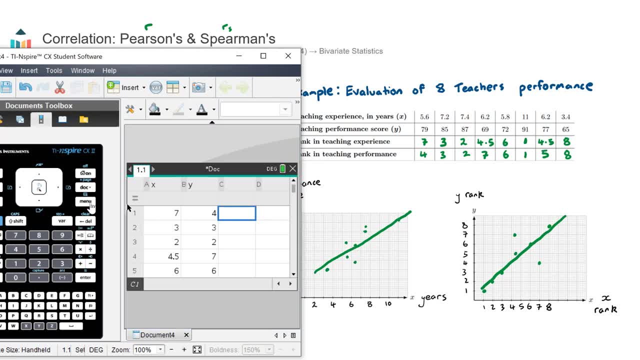 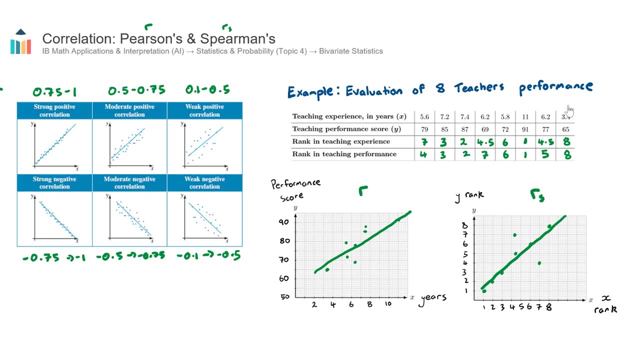 We then go ahead and perform a two variable stat calculation again. So, menu statistics, stat calculations, two variable stats: select X, select Y, And we get the RS value of 0.814.. Okay, so they are the two types of correlations. 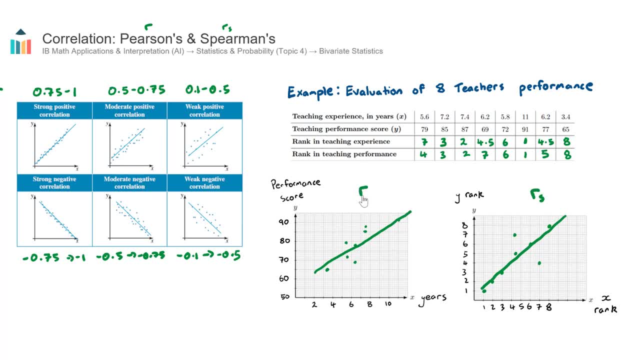 that you will need to understand in the AI course. We have the R value, which is based off the raw data, And then we have the RS value, which is actually based off the ranks of the data, And then we can describe the correlation. 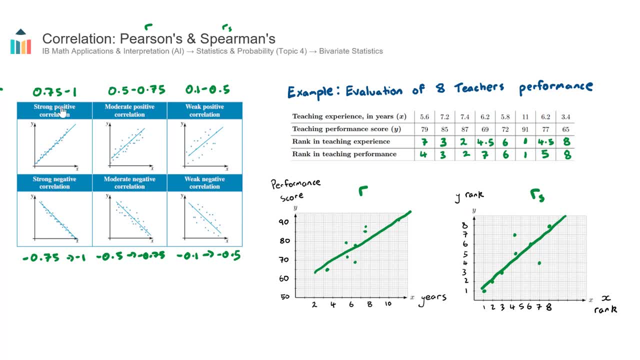 using these two descriptors here: either strong or negative, sorry. either positive or negative for the direction, and then strong, moderate or weak for the strength. Okay, that concludes our video on correlation.